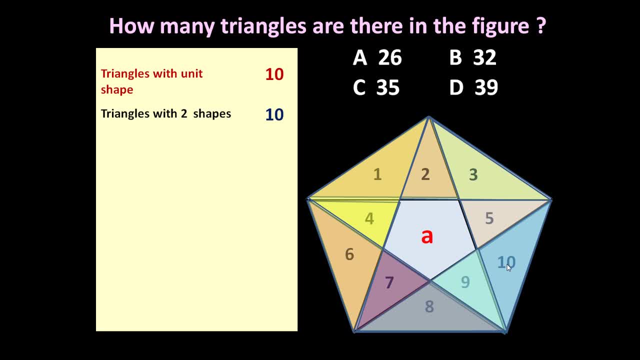 1,2,3,4,5,6,7,8,9,10. So, friends, 10 triangles are possible if we take two small shapes or 2 small may be to take 2 small shapes or 2 unit shapes together. 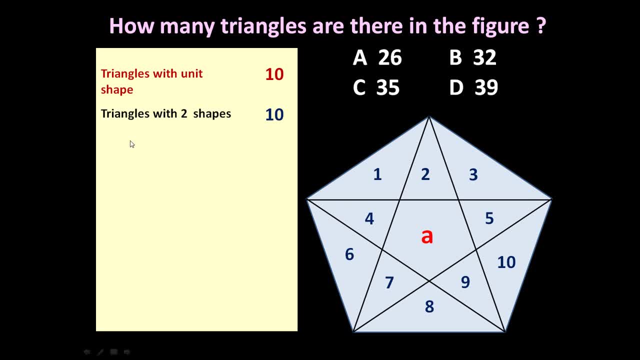 Friends, now let us count triangles with three unit shapes. If you see 3 unit shapes: 1,2,3, 1,, 2,3, 4, 5, 6. Now let us count the triangles with three unit shapes: 7,, 8,, 9,, 10.. So, friends, triangles with 3 unit shapes, 10 such triangles are possible. If we take just, you see, 1,, 2,, 3, it will form 1 triangle. 3,, 5,, 10, 1 triangle, 10,, 9,, 8, 1 triangle, 8,, 7,, 6, 1 triangle, 6,, 4,, 1, 1 triangle. 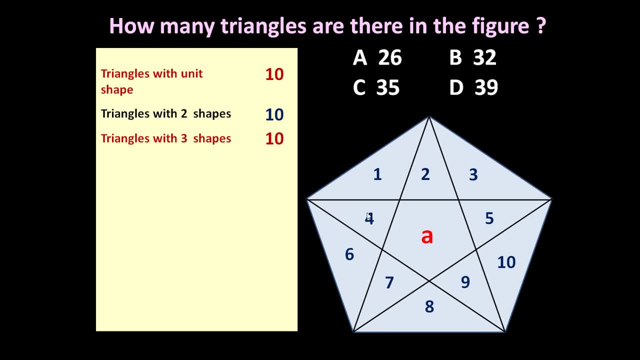 And other than these, if you see 4,, 5,, 8, 1 triangle, 2,, 9,, 8, 1 triangle, 4,, 5,, 8, 1 triangle 2,, 9,, 8,, another triangle, 4,, 8,, 9,, another triangle, 2, 7,, 8,, another triangle Like this, 5 more, So total 10 such triangles are possible with 3 shapes taken together. 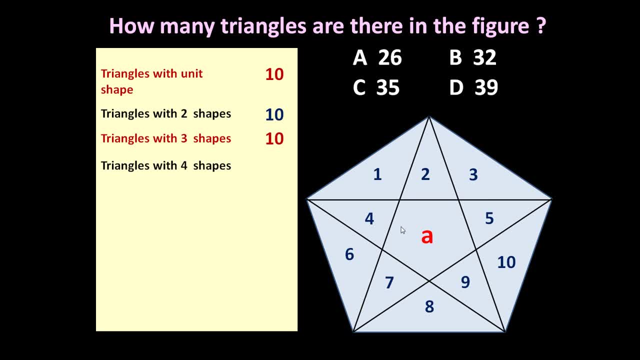 Ok, friends, if we take 4 shapes together, Any triangle will be possible. Any triangle can be formed if we take 4 shapes together. No, we cannot make a triangle if we take any 4 shapes together. If we take 5 shapes together, is it possible to make a triangle? 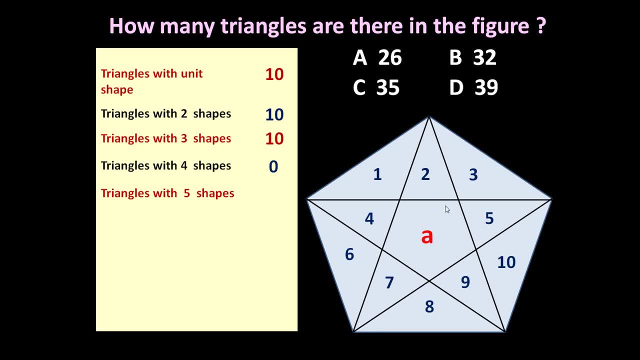 Yes, if you see 1,, 2,, 3,, 4, 5.. If we take these 5 shapes together, a triangle can be formed, And there may be some other: this, this, this, this, and this means 1,, 2,, 8,, 9 and 4.. 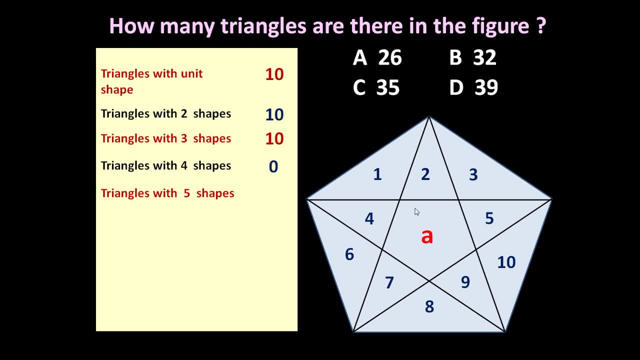 If we take these 5 together, a triangle can be Formed. So let us count 1,, 2,, 3,, 4 and 5.. So, friends, 5 such triangles can be formed if we take 5 shapes together.